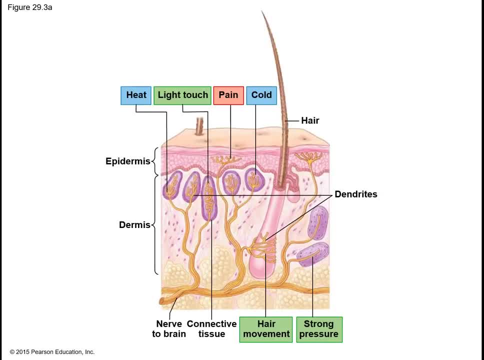 Here are images of the skin, of our skin, to give you an idea of how we are able to sense things. We have these receptors or neurons in our skin that will pick up on things like cold, pain, light touch or heat. Deeper still, we have receptors that pick up on strong pressure. 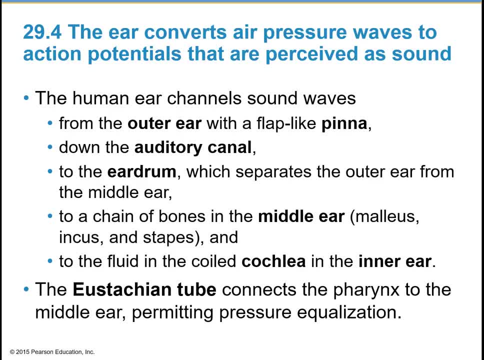 So looking into hearing and balance, first, The human ear channels sound waves: from your outer ear that has a little flap called the pinna, down the auditory canal, which would be your ear canal, to the ear drum which separates the outer ear from the middle ear. 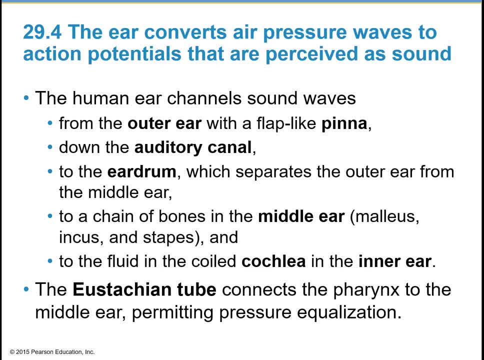 There's a chain of bones in the middle ear called the malleus incus stapes and to the fluid in the coiled cochlea in the inner ear. So we're going to take a look at all of that in a picture in just a second. 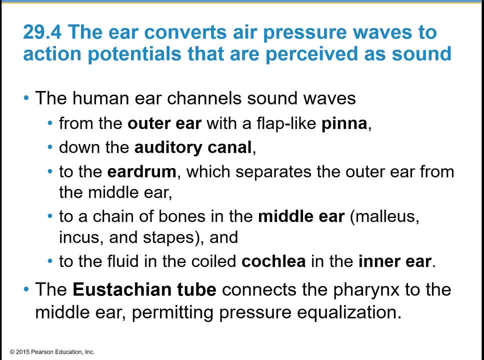 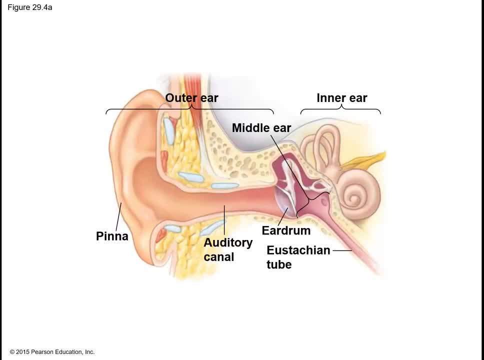 The eustachian tube connects the pharynx, which is the back of your throat, to the middle ear, permitting pressure equalization. So here's the outer middle and inner ear. So here's the outer ear that we see. 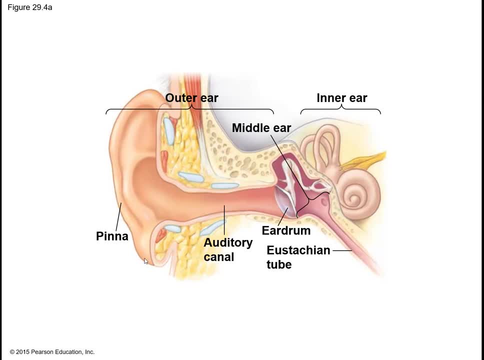 From the outside. this flap, known as the pinna, will channel sound waves down the auditory canal toward the ear drum. Behind the ear drum we have the three middle ear bones: the incus, the malleus and the stapes. 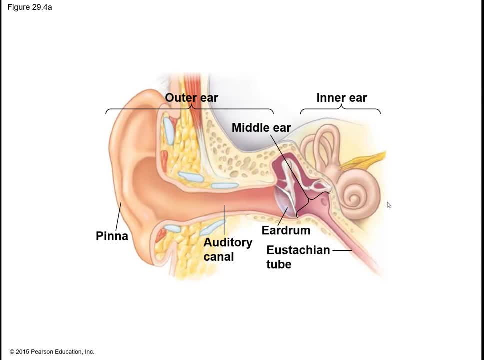 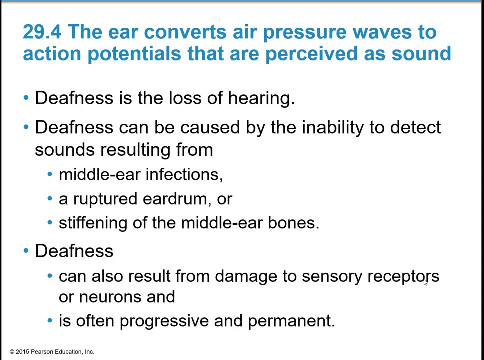 Then we have the inner ear, which has the cochlea in it. Here's the eustachian tube that will connect to the pharynx, or back of the throat. Deafness is the loss of hearing, and deafness can be caused by the inability to detect sounds. 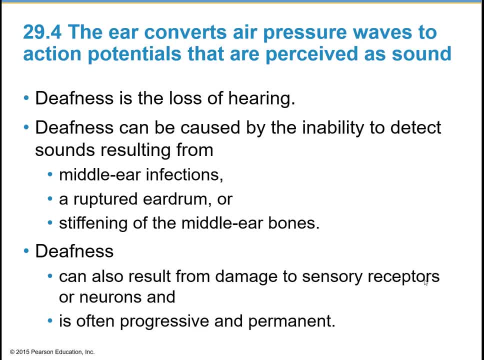 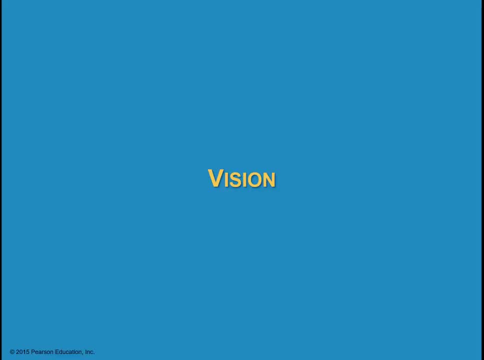 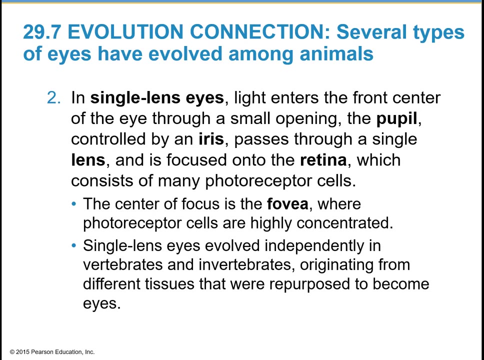 because of middle ear infections, a ruptured ear drum or stiffening of the middle ear bones. It can also result from damage to sensory receptors or neurons and is often progressive or permanent. Vision In a single lens. eye light will enter the front center of the eye through a little opening. 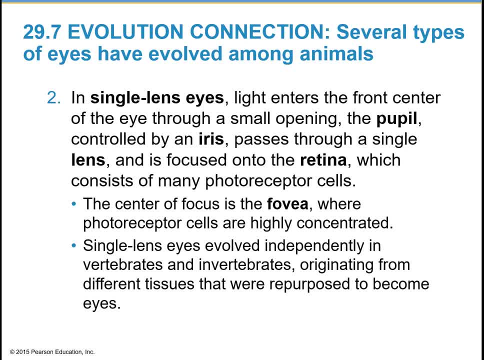 known as the pupil. The pupil is controlled by the iris, passes through a single lens and is focused onto the retina, which consists of many photoreceptor cells. The center of focus is the fovea. This is where photoreceptor cells are very concentrated. 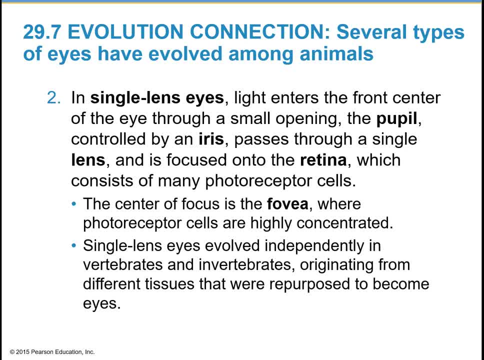 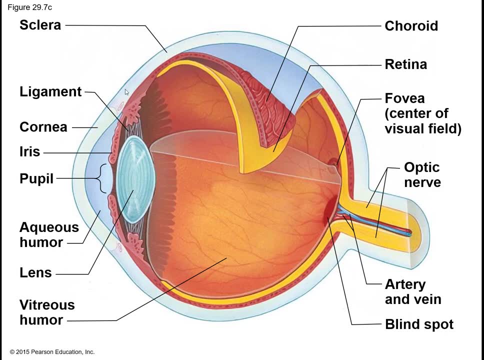 Single lens eyes evolved independently in vertebrates and invertebrates, originating from different tissues that were repurposed over time to become eyes. Here are the main features of a single lens eye. We have the white part of the eye, known as the sclera, which is very tough. then we have 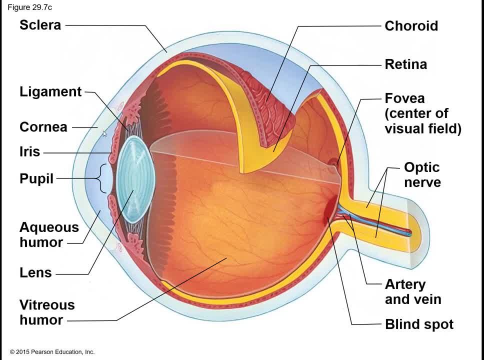 the cornea, which is a little bit more clear, and the cornea is going to cover up the iris, And the iris is the part of the eye that is colored either green, brown or blue. Then we've got the pupil, which is the black circle in the center of the iris. 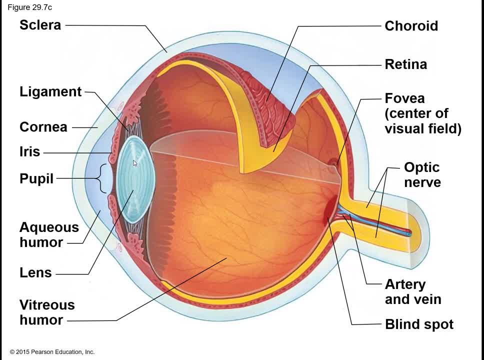 We have the lens and then in the very back, we have the fovea, which is the center of your visual field. The retina is here in yellow and the choroid is here in red. So retina and choroid, And then we've got our optic nerve which is going to carry. these receptors will carry. 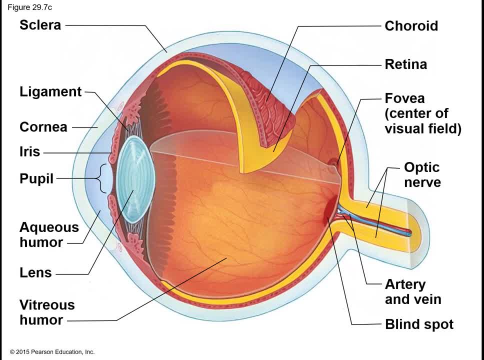 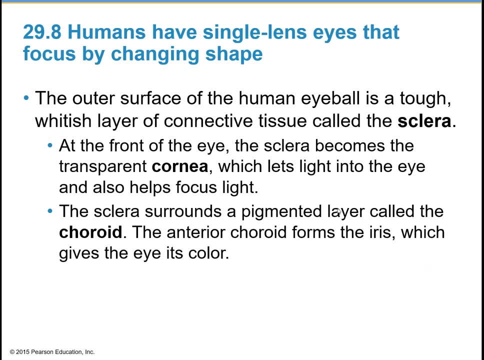 the signal to the brain so we can process what we see. The outer surface of your eye is a tough whitish layer called the sclera that we just looked at. At the front of the eye, the sclera becomes the transparent cornea which will let light. 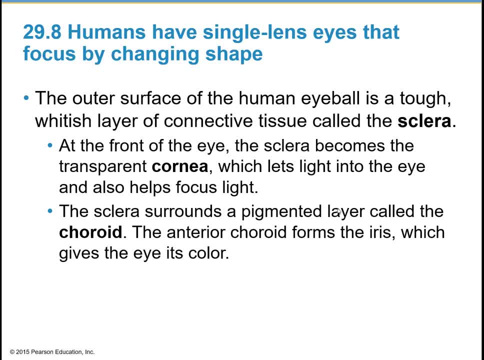 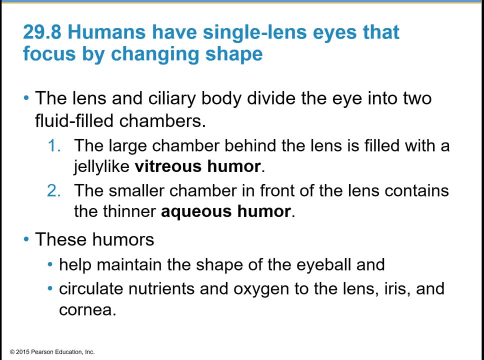 into your eye and also help focus the light. The sclera surrounds a pigmented layer called the choroid. The anterior choroid forms the iris, which gives the eye its color. In addition, we have two fluid-filled chambers. The large chamber, behind the lens, is filled with a jelly. 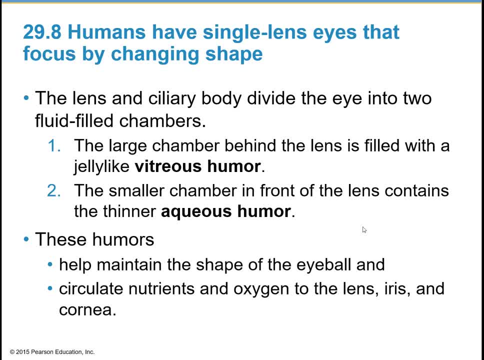 The choroid forms the iris which gives the eye its color. In addition, we have two fluid-filled chambers. The smaller chamber in front of the lens contains a jelly-like, vitreous humor, and the smaller chamber in front of the lens contains a thinner, aqueous humor. 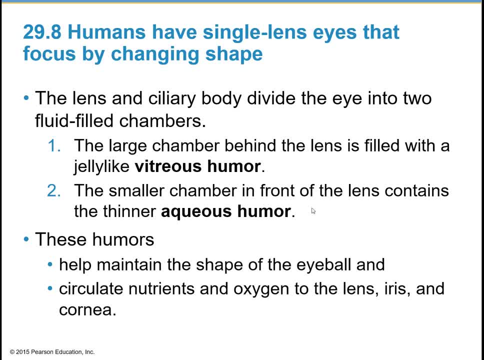 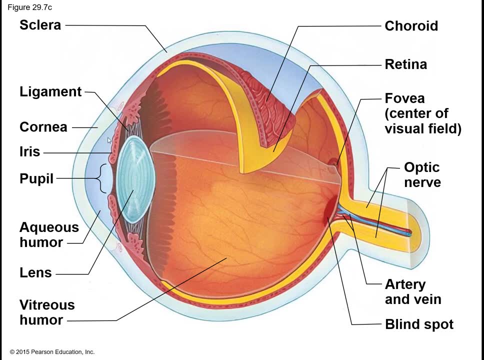 These humors are very important because they will help to maintain the shape of the eyeball and circulate nutrients and oxygen to the lens, iris and cornea. So, going back, we'll take a look at the aqueous humor which is right in here, filling this: 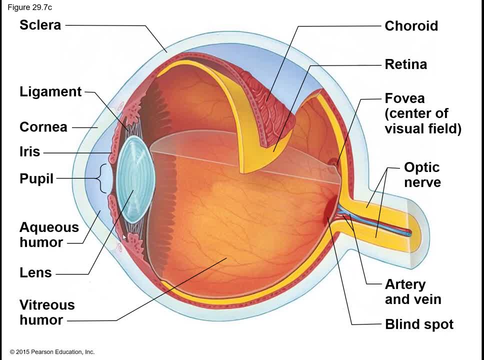 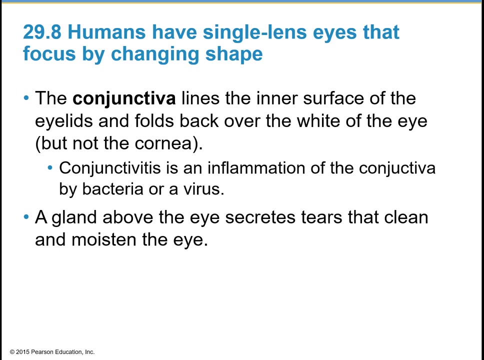 space under the cornea And then inside of the large cavity. we have the vitreous humor giving the eyeball its shape and also circulating nutrients and oxygen to the lens, iris and cornea. The conjunctiva lines the inner surface of the eyelids and folds back over the white. 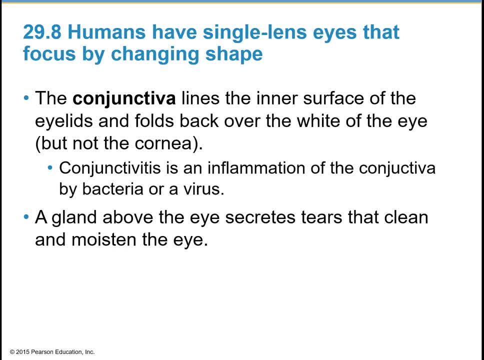 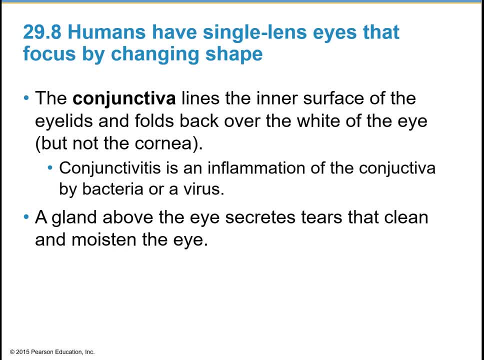 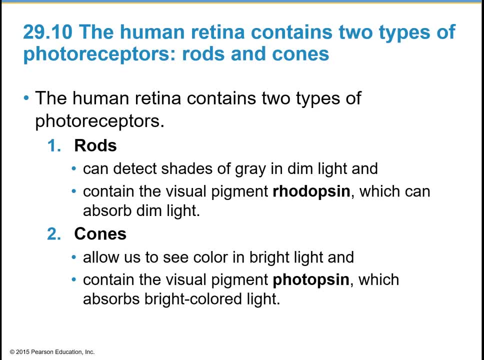 Conjunctivitis is an inflammation of the conjunctiva by a bacteria or a virus. A gland above your eye secretes tears that clean and moisten the eye. The human retina contains two types of photoreceptors. We have rods and we have cones. 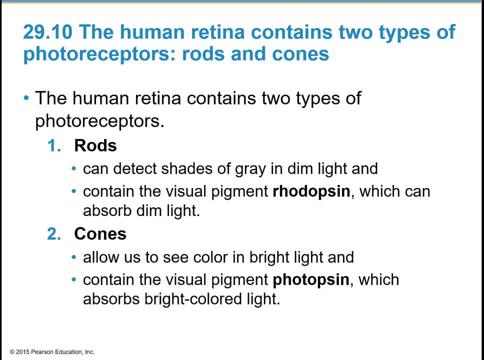 Rods are what will detect shades of gray in dim light and contain the visual pigment rhodopsin, which can absorb dim light. dim light Combs will allow us to see color in bright light and contain the visual pigment bodoxin, which absorbs bright colored light.